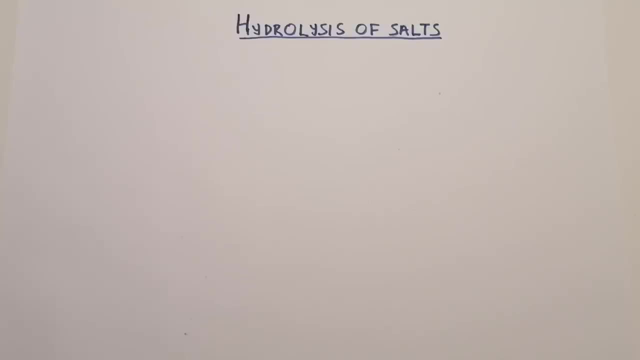 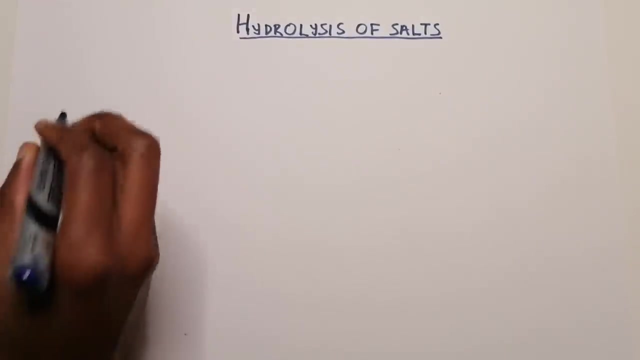 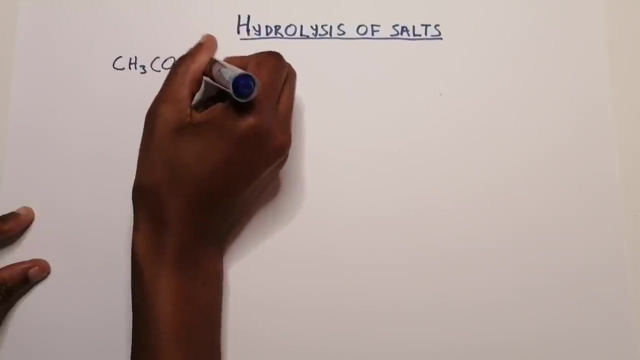 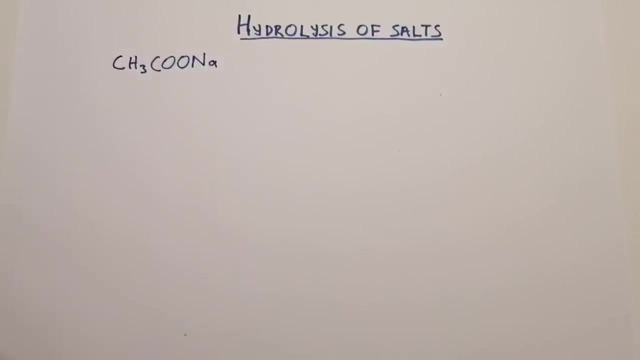 Acidic basic or will it be neutral? okay, Now I'm going to take a couple of examples. let's say, for argument's sake, they give you something like sodium ethanoate, which is something like CH3 COONA. okay, something like this. They give you the salt and they want to know if this salt is. 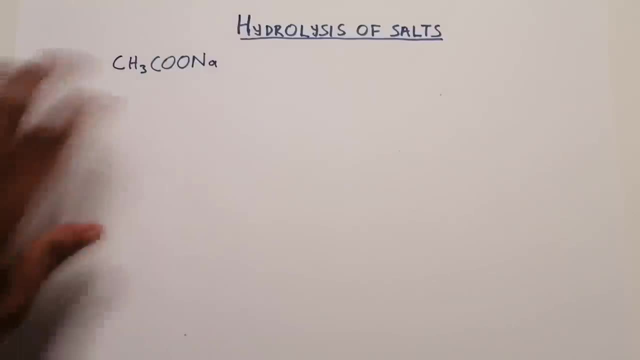 acidic or basic, or rather the resulting solution. So meaning that if they take the salt and put it in water, will the resulting solution be acidic, basic, or will it be neutral? okay, I'm sure you've seen those questions and they would therefore say to you: prove by means of a reaction. okay. So I want to show you that. 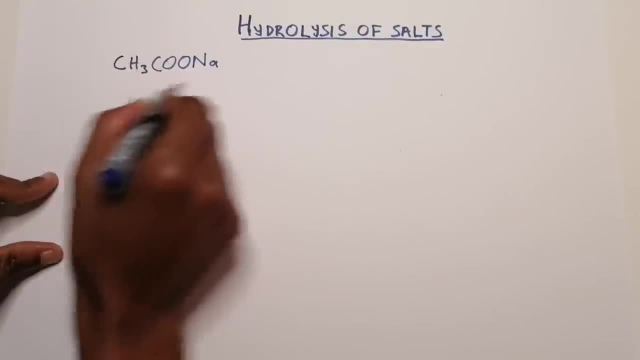 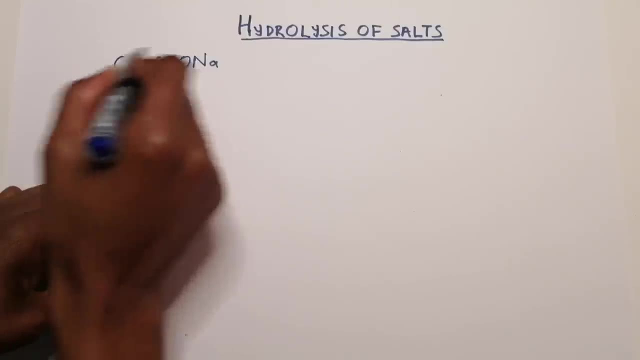 quickly. So what we do here is that we simply take this salt as it is right, and I want us to find out: where does this salt come from? So I'm going to take this salt and I'm going to put it in this reaction. So they say that this is what salt actually come from. I want you to think about it. 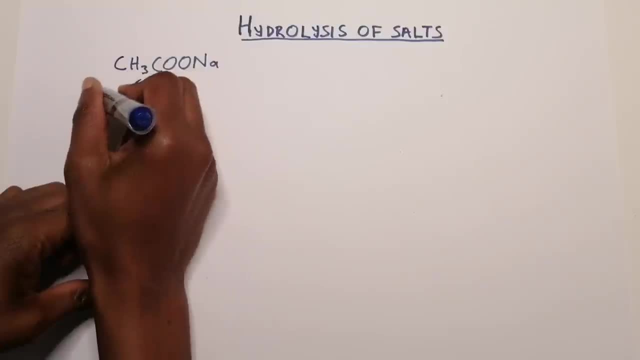 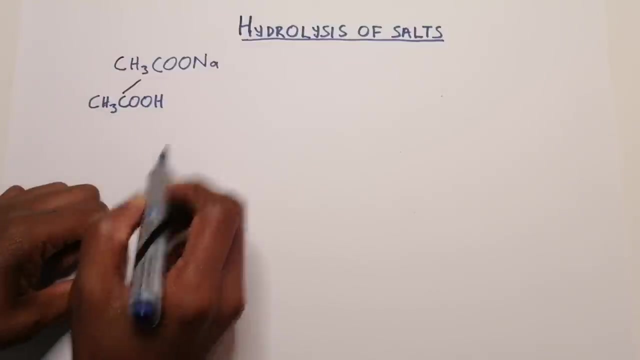 CH3 COO. this would have come from CH3, which acid and base reacted to give the salt. So it's CH3 COOH. this is ethanoic acid. So this portion here comes from ethanoic acid, isn't it? Sodium, usually this guy comes from what? from sodium hydroxide. Okay, so, in order to produce 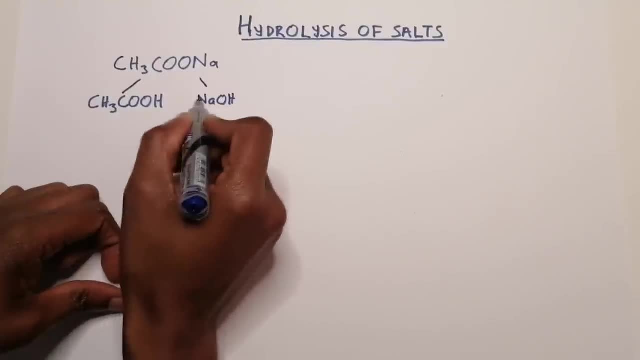 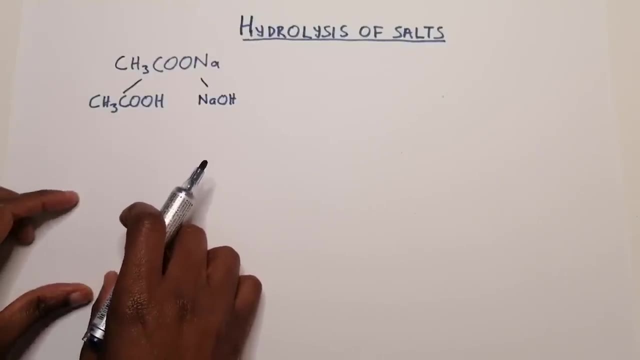 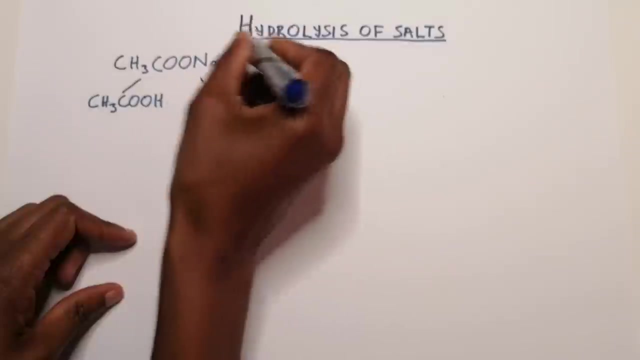 the salt. we need to have some extra oxygen, okay, So I'm going to take this salt and I'm going to. it means that you took sodium hydroxide and ethanoic acid, or what we term acetic acid. okay, now what we're going to do is let's first ionize, or, um, you know, um, let the salt undergo. 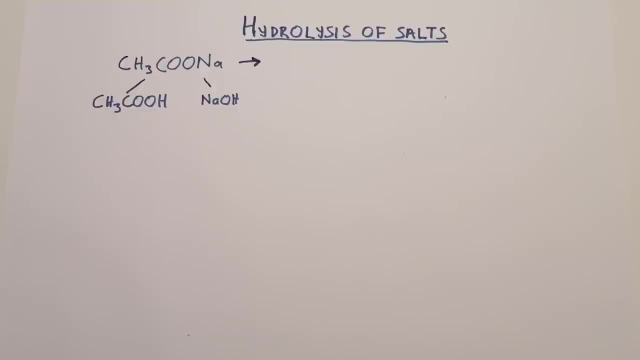 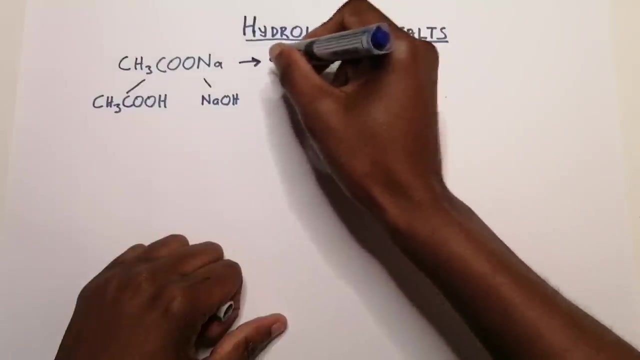 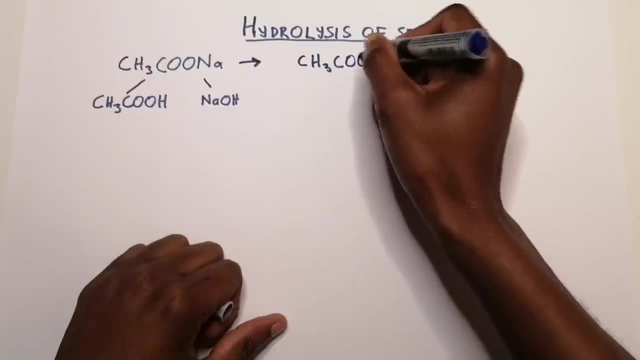 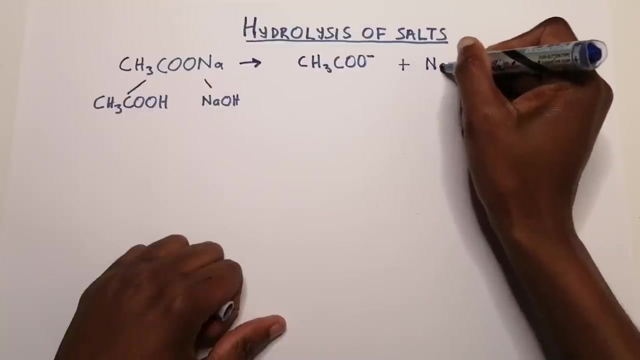 um, or dissociation, right um, so it will. the salt will undergo dissociation, right? so in this case you'd have, if it dissociates, you'll have ch3 coo minus. now, you should learn this. uh, if you know, don't know where this comes from, just learn it off by heart if you have to. okay. so when this 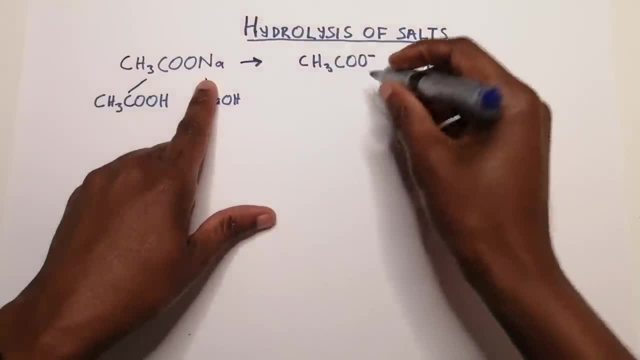 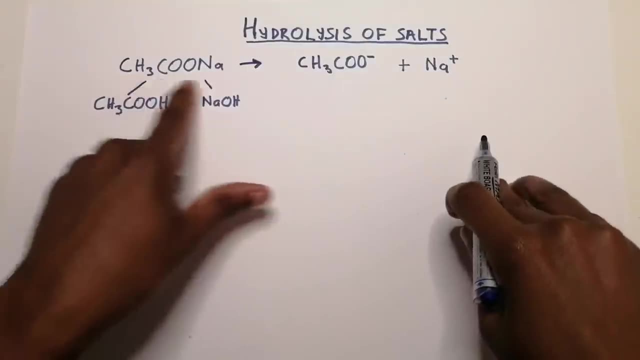 guy breaks down: you've got two things that you're going to have to do, okay, so you're going to have form there. you've got the ch3, coo minus portion of it and you've got the na plus portion of it. okay, that's where this guy comes from. now, ladies and gents, i want you to please listen carefully. 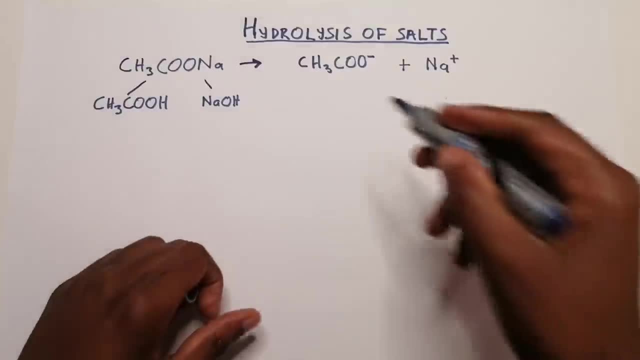 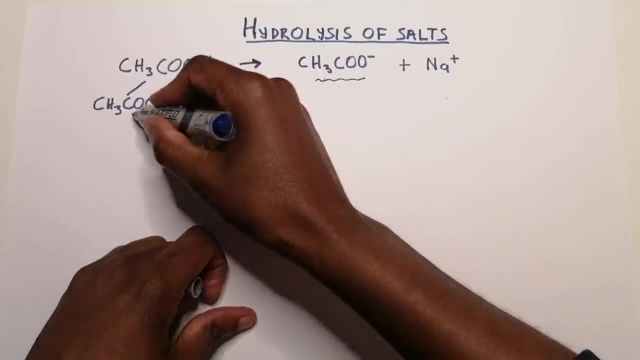 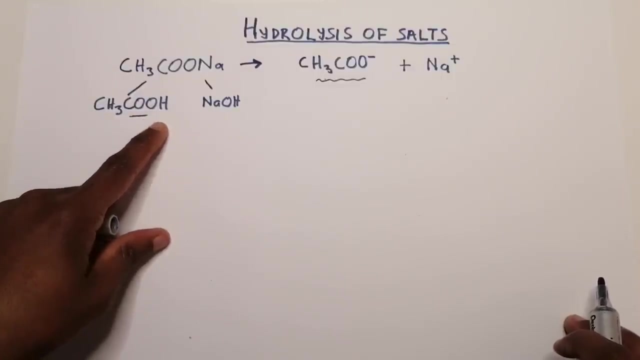 okay, so i'm going to show you where does the ch3 coo come from? okay, where does it come from? it comes from this acid over there, ch3 coo h, which is ethanoic acid. okay, so what type of acid is this? now, remember what i said to you: there are three strong acids that you have that sulfuric. 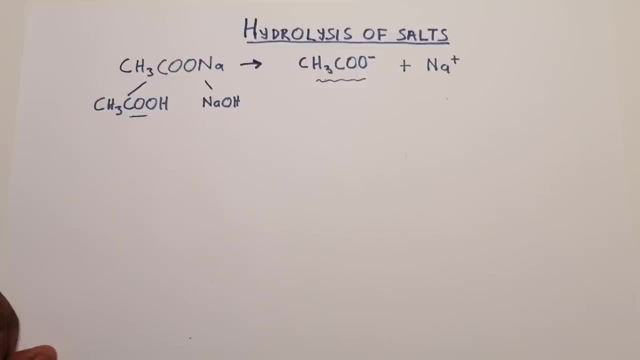 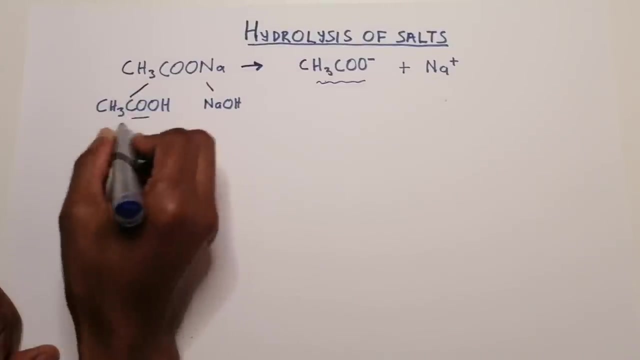 acid, hcl, hydrochloric acid, sulfuric acid and nitric acid. so anything out of those right is really considered to be a weak acid. so therefore, of course, every organic acid, by the way, is a weak acid. so this guy comes from a weak acid. so we know this guy is weak, okay, so now? 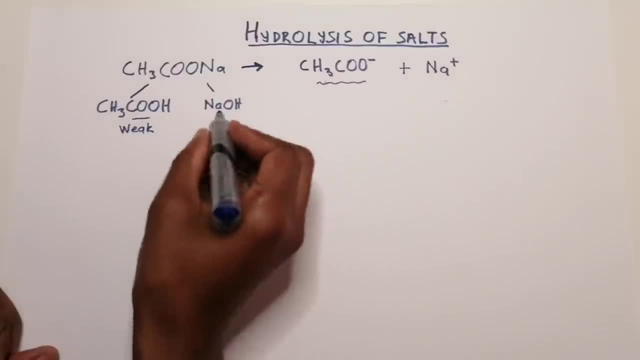 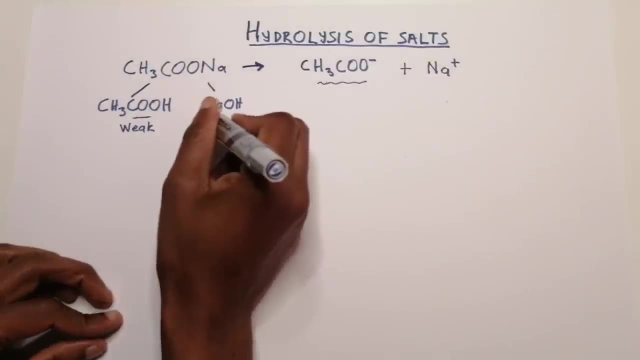 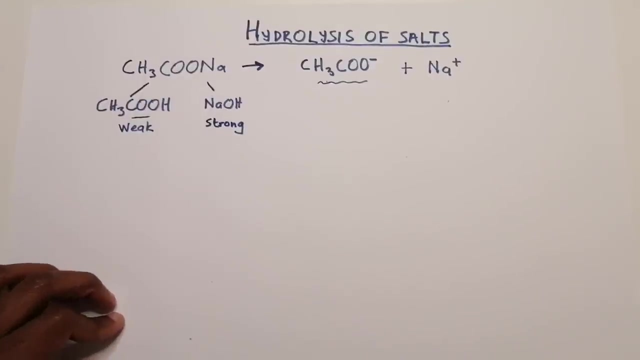 we know what type of base is this. so sodium hydroxide and potassium hydroxide, those are relatively strong. okay, so we consider this guy to be a strong base. okay, so sodium hydroxide. now, if you don't know this, please just watch the other videos on. 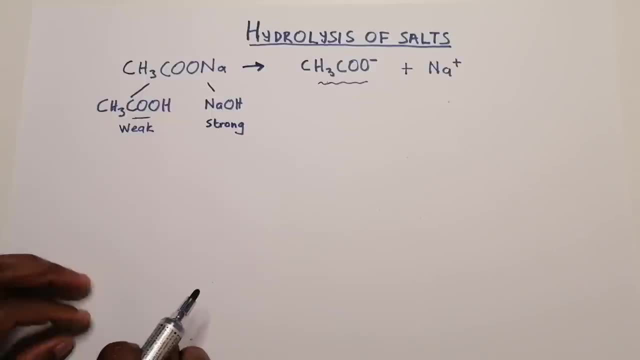 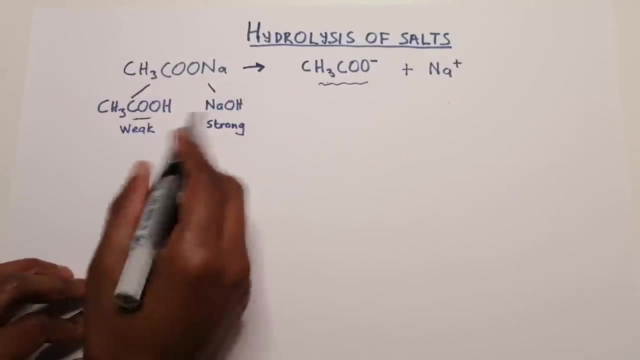 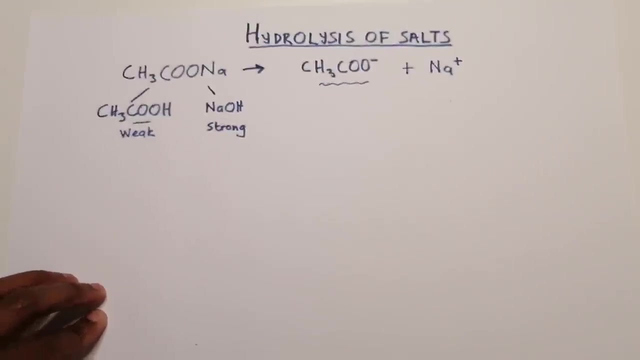 acids and bases, and you should be able to at least get up to speed with that, right. so we say this is a strong base and that's a weak acid, all right. we said on the basis, remember, it's just sodium hydroxide and potassium hydroxide. of course you've got all the other hydroxide bases. 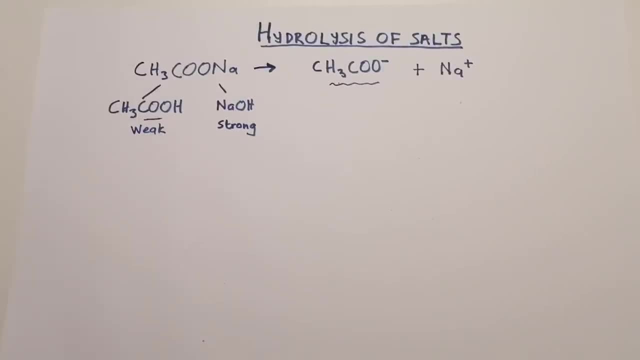 um, but of all those sodium hydroxide and the potassium hydroxide and potassium hydroxide are the strongest. right now i'm gonna prove whether this would be a, an acidic, or a- uh, a basic solution. okay, when we put it in water. whether, when we take the salt and put it in water is it is that. 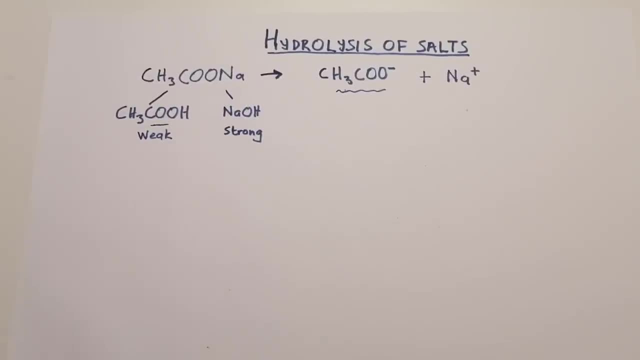 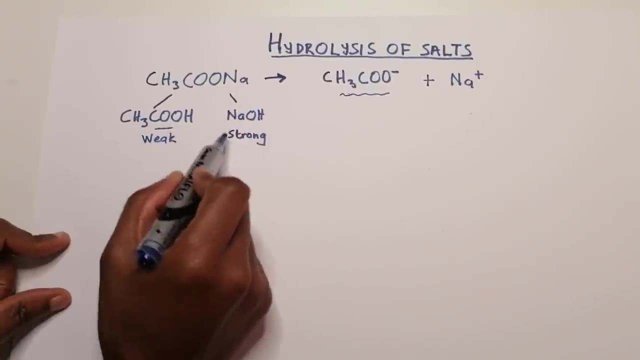 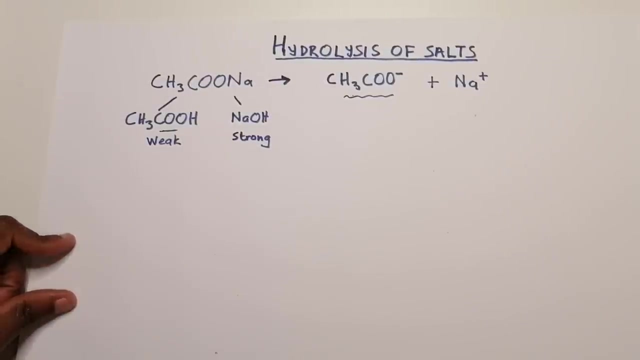 our resulting solution going to be acidic, basic, or is it going to be neutral? now, look at this. you've got a weak acid that reacted with a strong base. who's winning the game right now? you've got a in this relationship. definitely it's the strong one, right? so definitely it means that the resulting 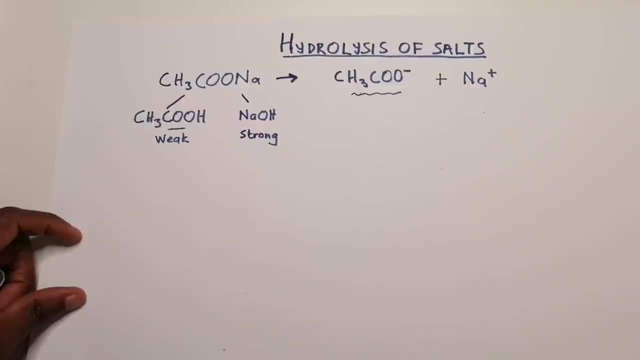 salt, which is this guy here- is going to be basic. okay, all right. so when we put it in water, the resulting solution will be alkaline, isn't it? it will be a basic solution, right? so, as a result, how do i now prove that? with a reaction, all right, so i was just showing you here how you get to the weak part. 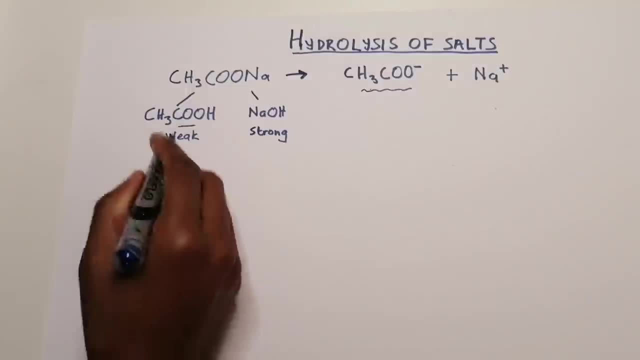 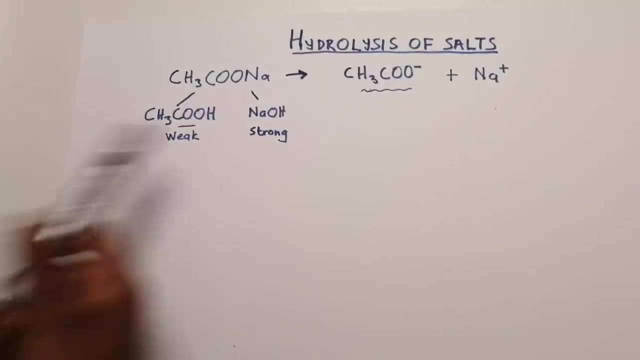 and the strong part. so i already know, from what i've just shown you here, i already know that the resulting solution will be basic. why? because it was the reaction between a weak acid and a strong base. so therefore this guy would dominate and, as a result, the resulting solution will be alkaline. 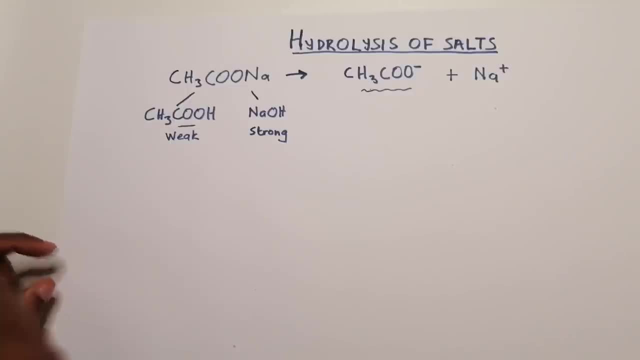 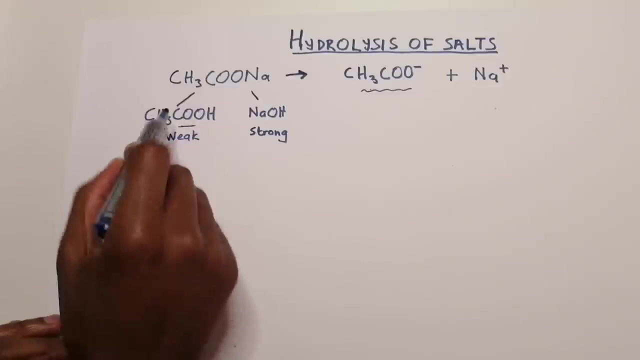 but now let's prove it. okay, how do you know? how, then, do you use an equation to prove that? you'll always look at the two things that reacted right and you simply say to yourself: okay, a weak acid will always give rise to a strong conjugate. now, please note this. this guy came from that, so this guy is weak, so meaning. 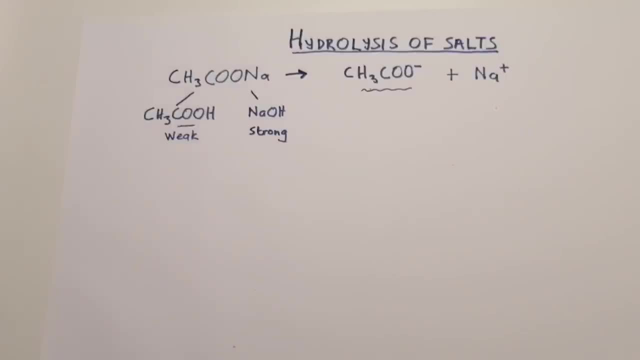 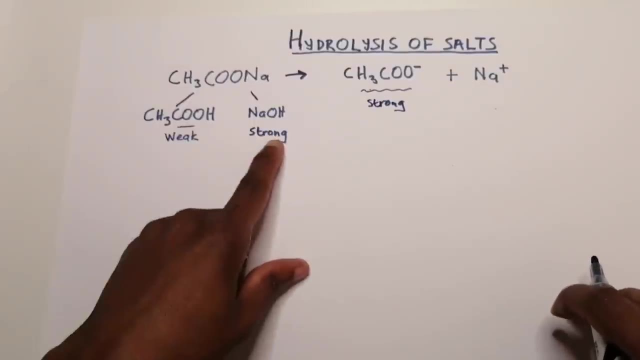 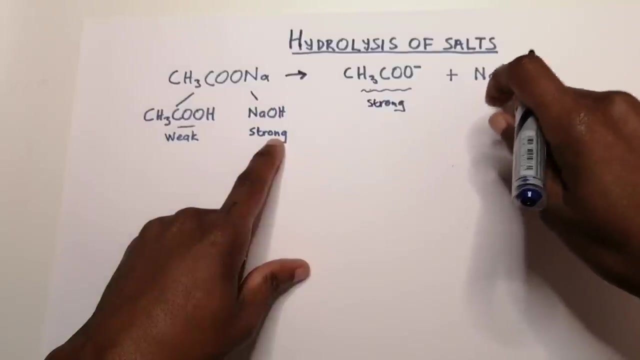 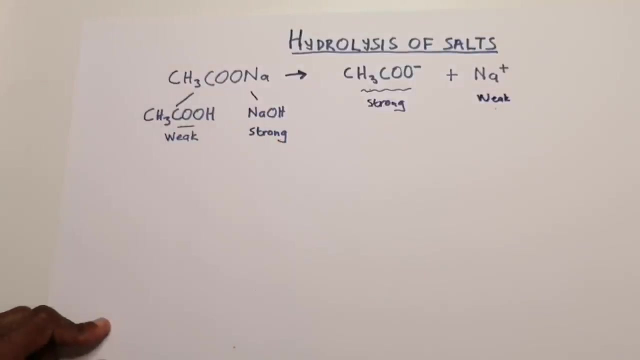 that the conjugate is all is, is is strong, so this guy would therefore be strong. okay, this is a strong uh base, right? it means that the iron there should be weak. so, as a result, this guy is weak. okay, so now all you simply do to prove that this salt here will result in a basic 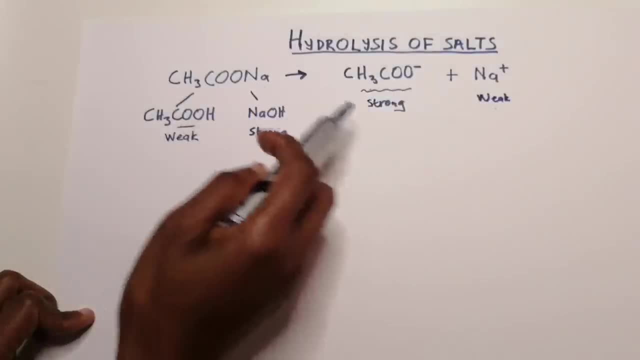 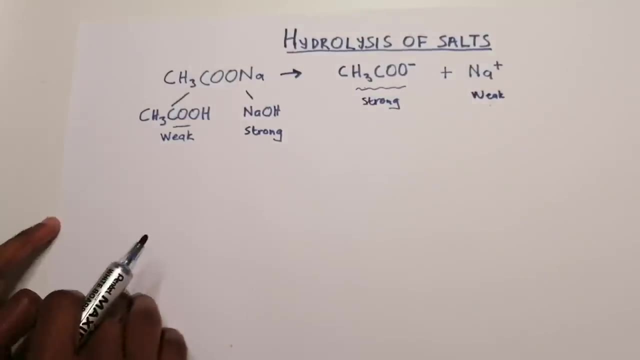 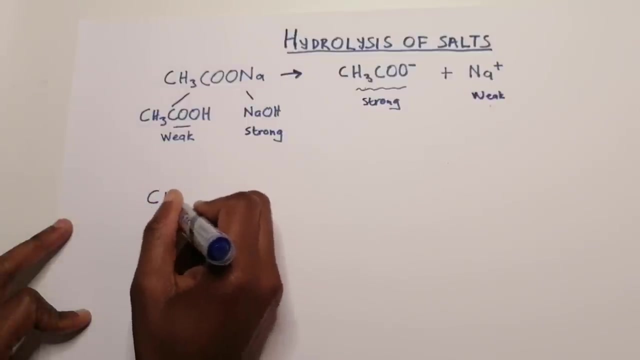 solution. all you do is you always take your strong iron. okay, you'll see when we do the next one. okay, you take the strong iron and you react it with water. so let's take the strong iron. which one is the strong iron? of course, that one, right. so it's going to be ch3, coo minus, and then i'm going. 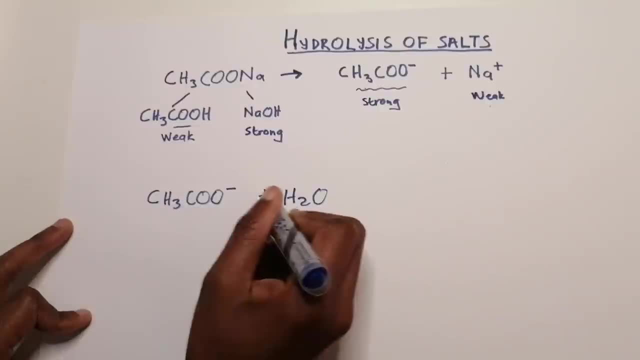 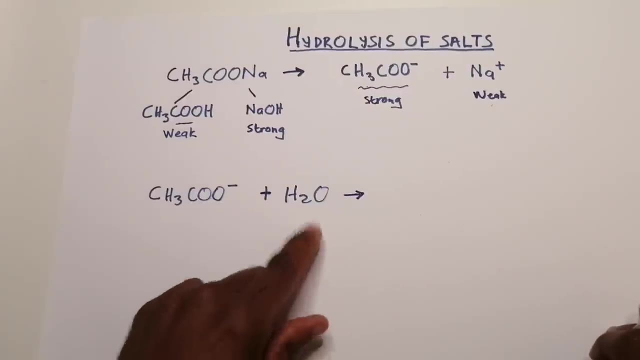 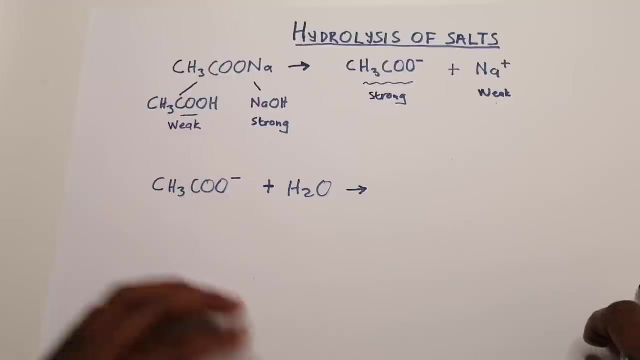 to react it with h2o. okay, and what do i end up with? okay, strong iron, and i react it with water. so this is the actual proof here. i was just explaining to you how you can react it with water. you get to see which one is the strong or the weak. so we take the the strong iron, react it with water. 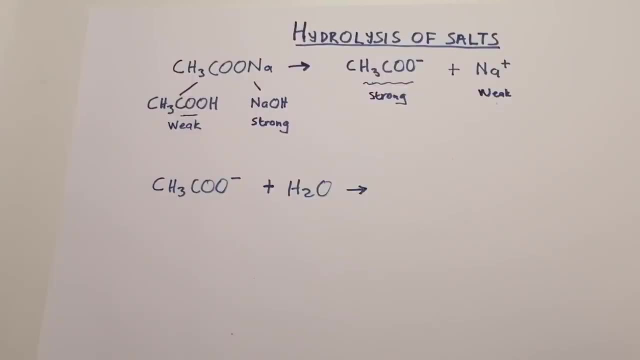 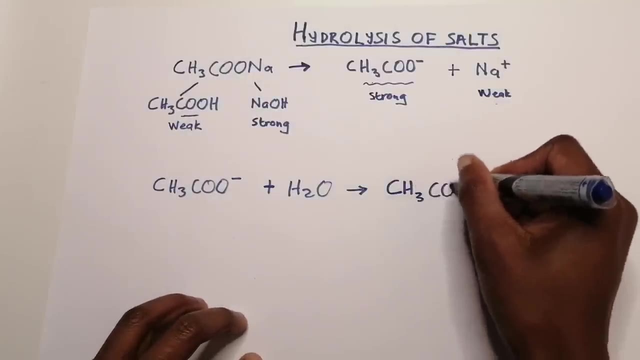 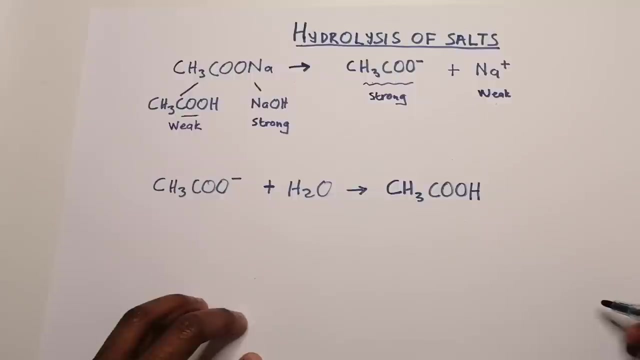 so it's the strong iron that always reacts with the water. okay, right, and what do we now have? we're going to have, as a result, ch3 coo. now, water is going to simply donate there and we end up with an h right. so ch3 coo, h. so 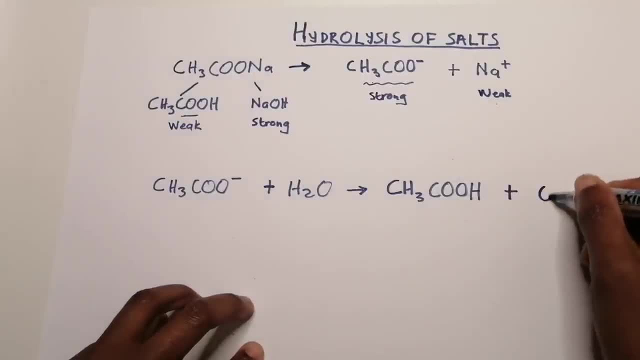 now, what have we done? we now have, oh, minus over there, okay, and notice, the presence of your hydroxide ions means that the resulting solution will therefore be alkaline or it will be a basic solution. okay, right. so just to quickly recap, what did we do? we simply took, okay, a salt, so they gave. 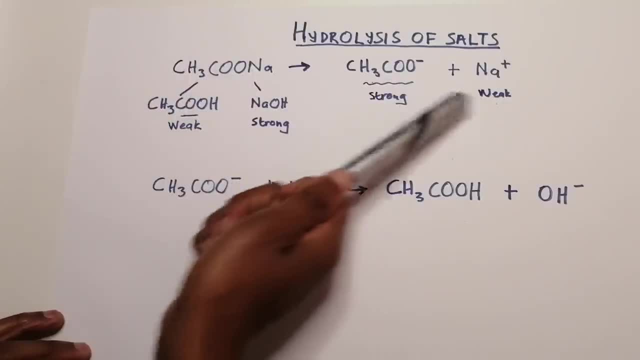 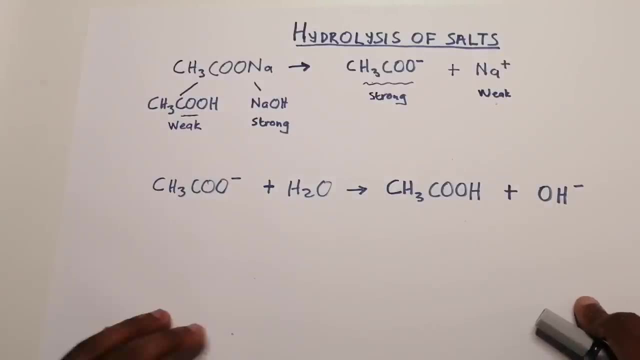 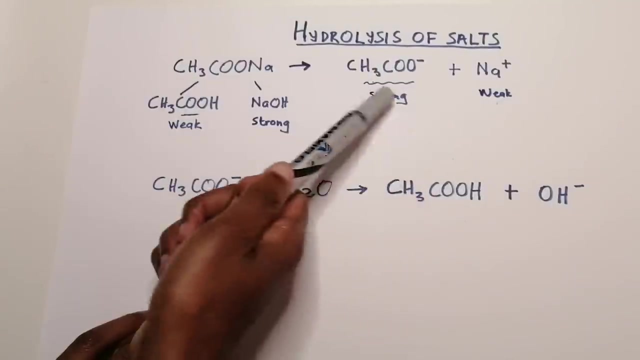 us the salt. we said: the first thing that you do is to ionize that salt or to make it undergo, um yeah, ionization or dissociation, right, and then all that we simply did. when it undergoes dissociation, we identify which one is the strong one, based on where it comes from, right, okay, we 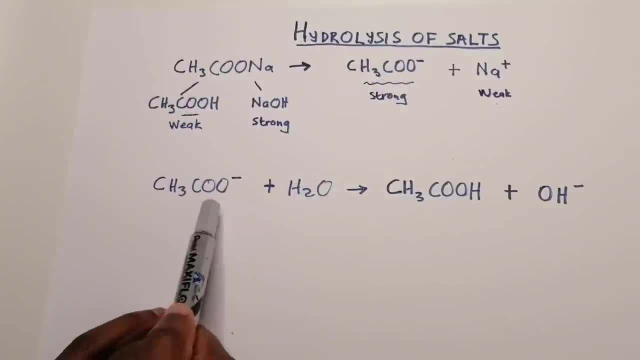 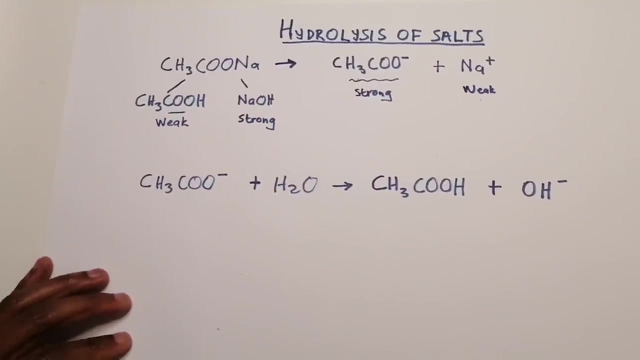 identified. this guy is strong. so therefore, the strong ion reacts with water and, as a result, you look at the um, the, the ion that results in that case and that will tell you whether it is an acidic solution or a basic solution. let me show you with another example so that you'd see. 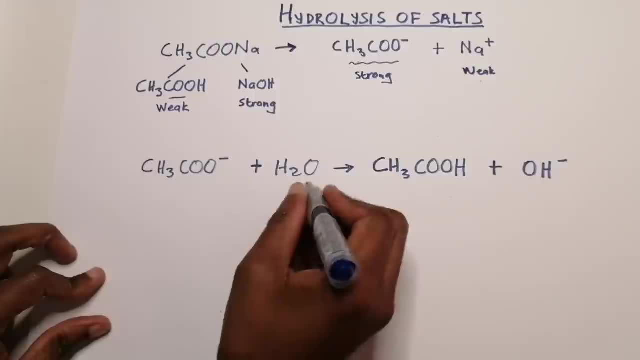 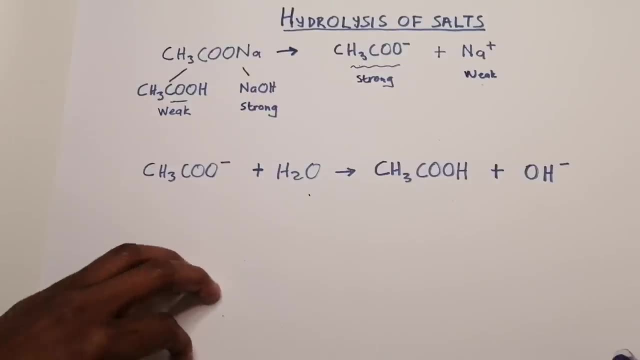 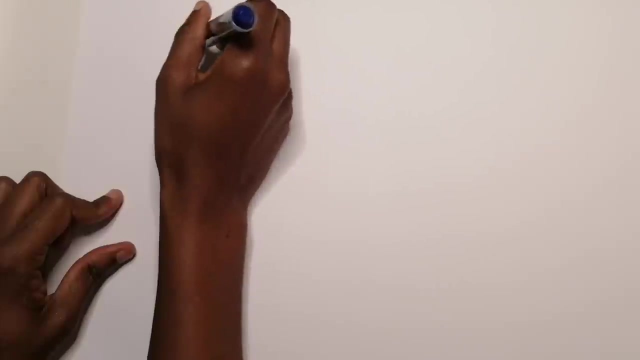 how i'm going to do that very quickly. right, let's take for argument's sake: you've got ammonium chloride. okay, right, in fact, let me do that in a in another sheet, right? so let's say, we've got ammonium chloride, so ammonium chloride looks something like this nh4cl, right? okay? so when 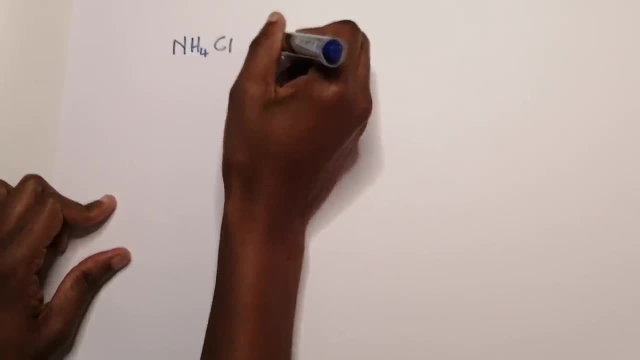 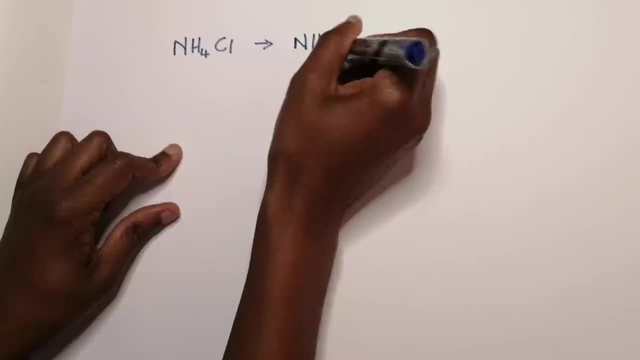 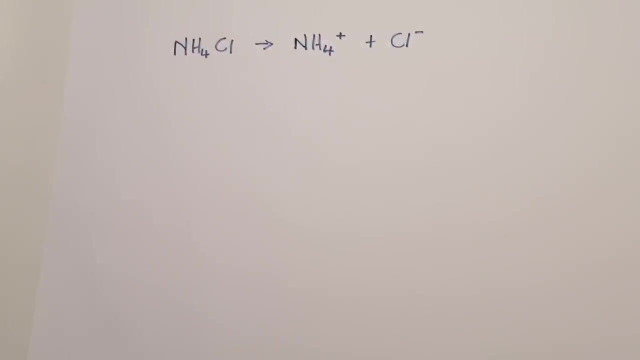 we take ammonium chloride, where does it come from? okay, so when we dissociate this guy? okay, so it will be nh4 plus plus cl minus. ladies and gents, you can either do this question in one of two ways. okay, it's: either you take my videos and you remember this stuff, okay, or you you try to. 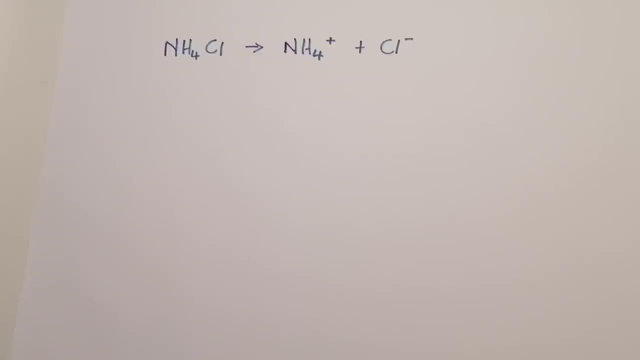 understand it. either way, it works okay and you'll still be able to get full marks. so ammonium chloride. so we want to prove whether the resulting solution is acidic, basic, or will it remain the same, okay, i mean, or will it remain neutral, okay. so now we need to find out once again: where does ammonium 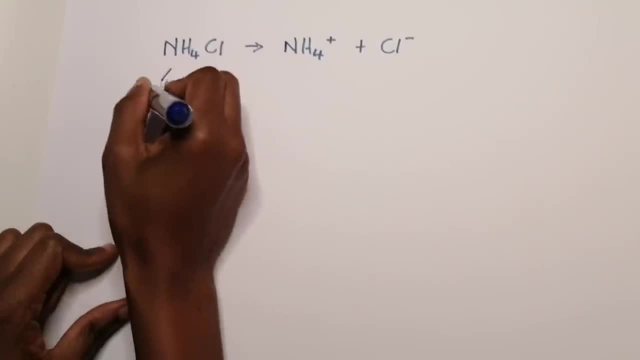 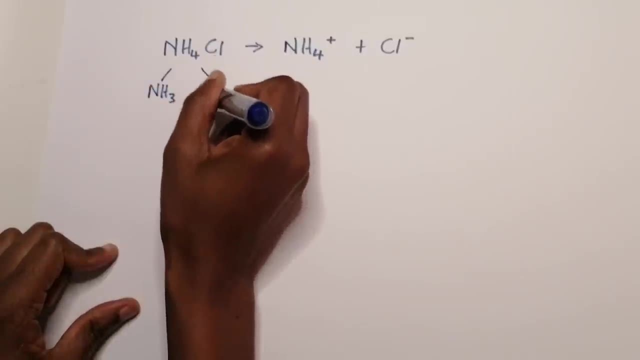 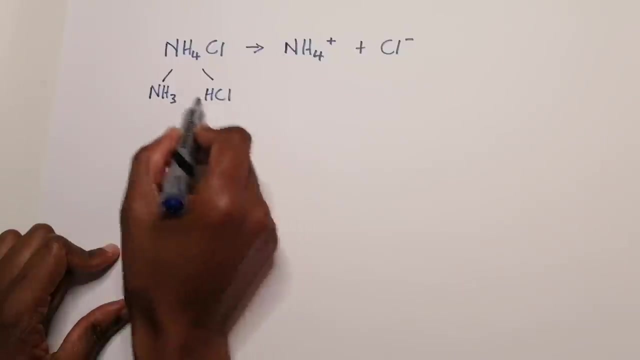 come from. so it means here we reacted two things. we reacted nh3 ammonia with hydrochloric acid. okay, so now remember what we said. so what type of a? so this definitely is an acid. this guy is a base or alkali right. so in this case we're saying: all right if we took nh3 ammonia, right, which is a base right. 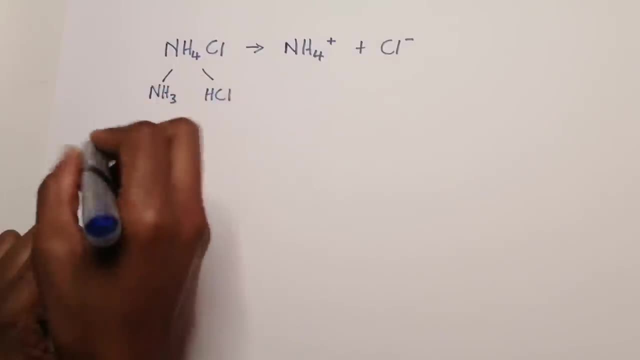 so in this case, what type of a base is this? we know it's not sodium hydroxide, it's not potassium hydroxide or any of the hydroxide bases. so in this case this guy is weak, so that's a weak base, okay. and what do we know about hydrochloric acid? remember we? 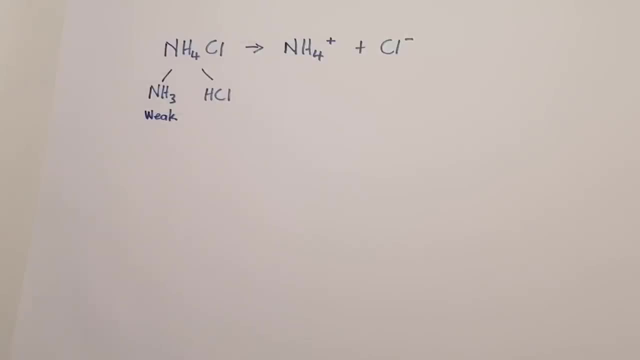 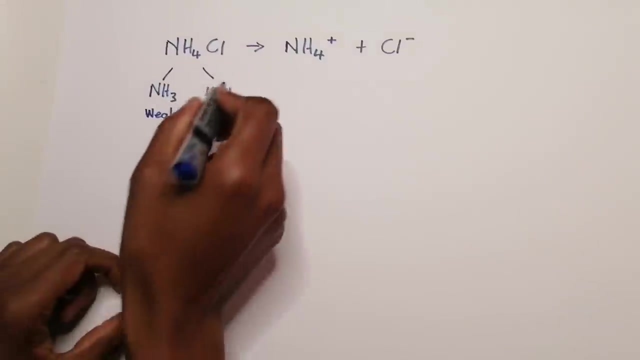 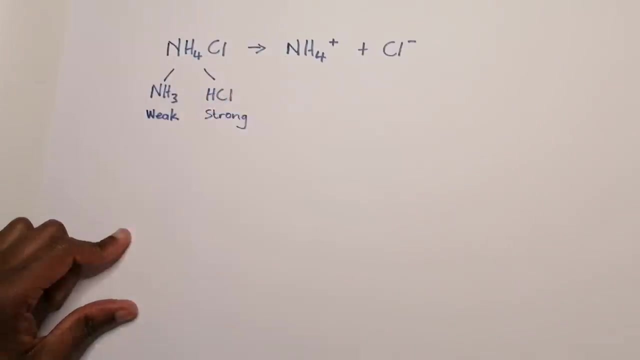 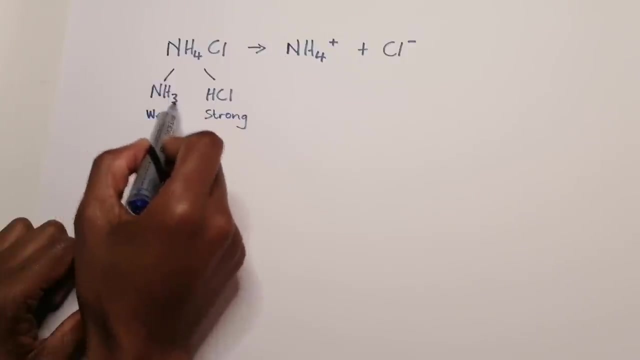 said we've got three strong acids: hydrochloric acid, as well as uh high as sulfuric acid, h2so4 and nitric acid hn03. so definitely that guy is a strong acid, so that's a strong acid, okay. so look at that. so we said a weak acid, a weak base, rather will give us a strong conjugate. 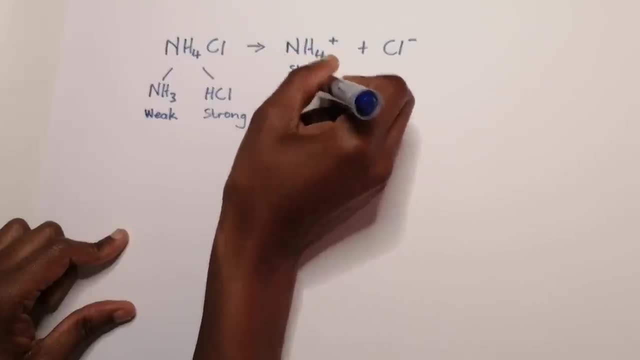 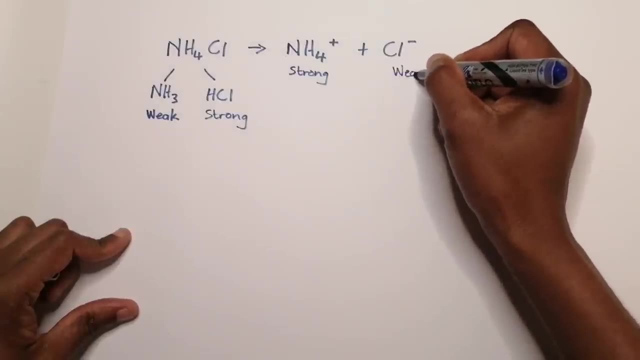 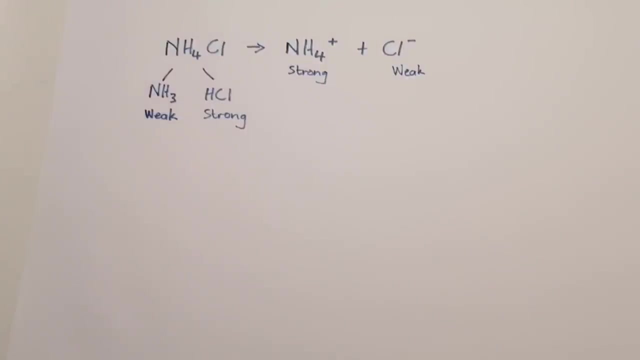 so definitely, this guy is strong, all right. and then we've got a strong acid there. it gives us a weak conjugate, isn't it okay? so we said you always take. now we're going to prove: is ammonium chloride okay, going to be, uh, when we put it in water? 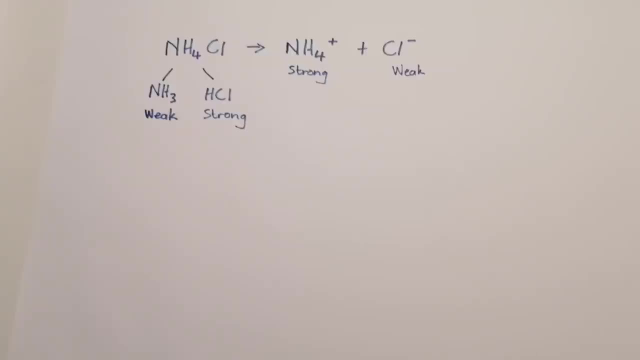 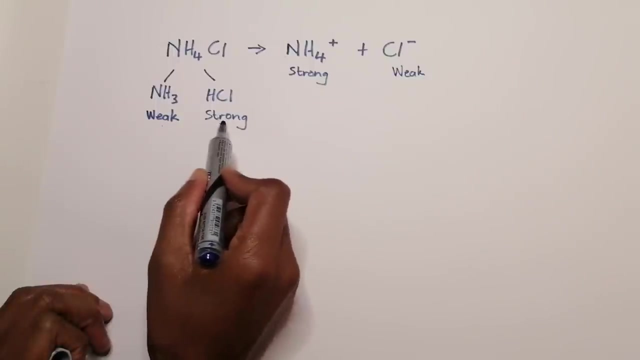 is it going to uh the resulting solution? is it going to be acidic, uh, basic, or will it remain the same? so all that we simply say, okay, look at this, i'm going to answer it before we actually do the- the resulting solution. so it's a weak base with a strong acid. who's winning there? definitely the 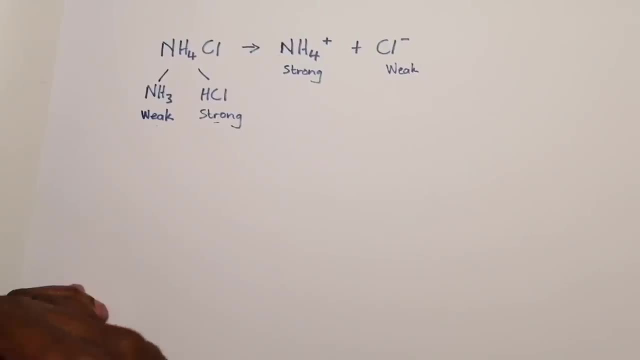 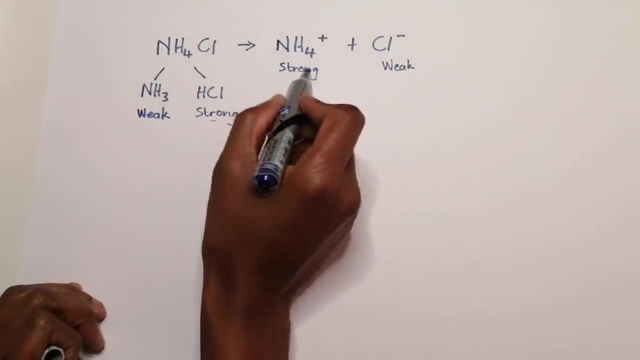 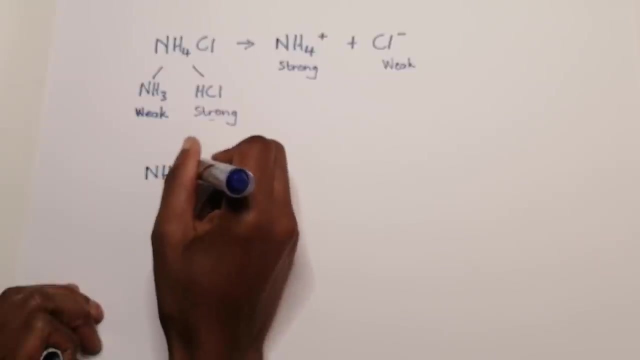 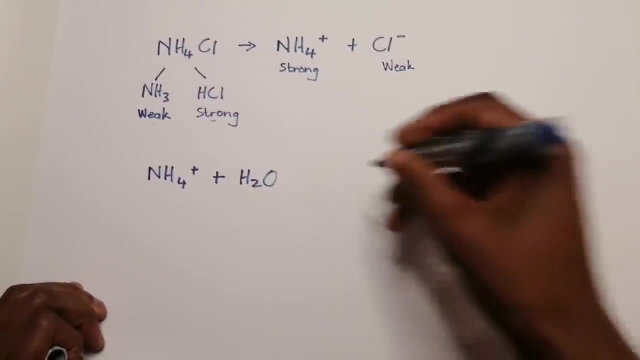 acid is dominating, so it means the resulting solution will actually be acidic. but let's prove that now. okay, now, remember, we said we take the strong conjugate and we react it with water. so i'm going to take nh4 plus. it's the one that's going to react with water, h2o, and what does it do? okay, 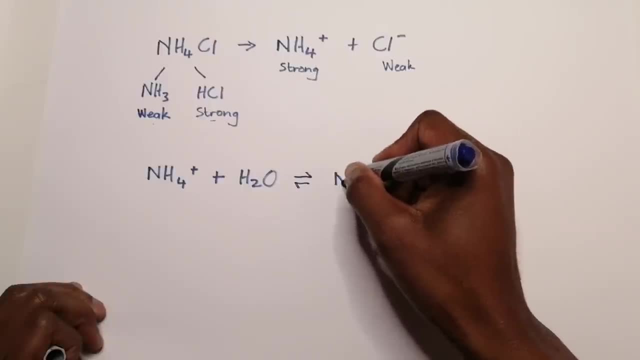 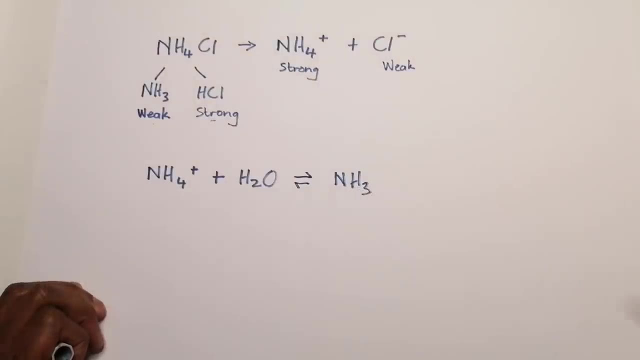 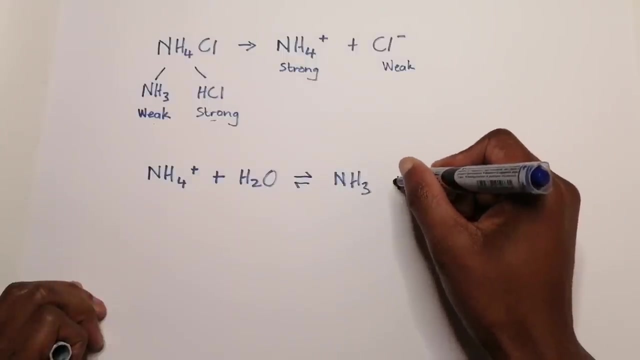 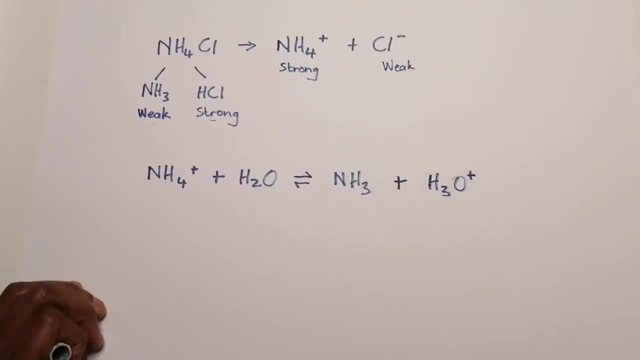 what do we get? we will get and h3. please note, there's no nh5 plus okay. so what will form is nh3. so what would have happened? it means this guy would have donated, uh, h plus okay, to water. so what would you have? on the other side, that's h3o plus okay. so, as a result, what do we notice? 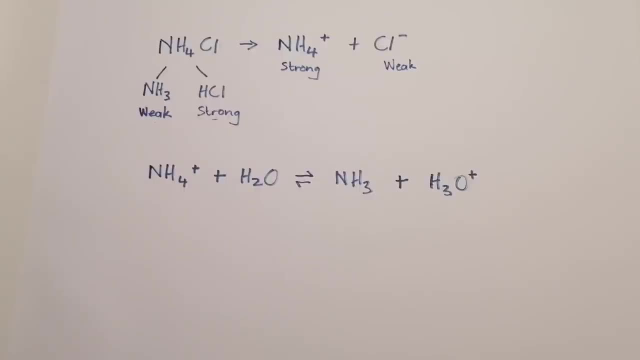 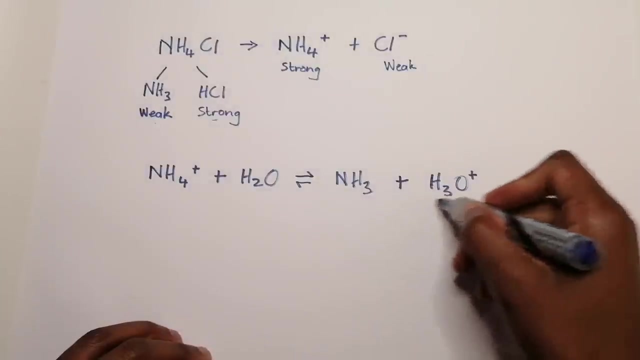 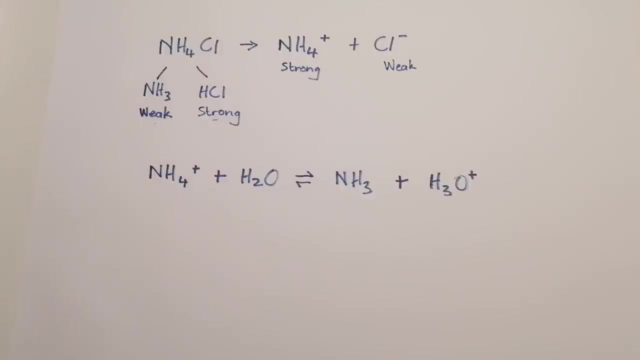 we've got h3o plus on the other side, so it would simply mean that the resulting solution is acidic and we've proven that right. why? because of the presence of our hydronium ions. okay, right, so that is how you would prove that there, okay. 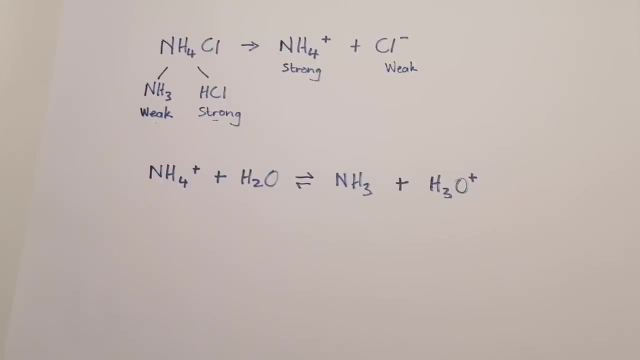 so i hope that has been helpful. that is how you actually um do the hydrolysis of salts. okay, and i hope that has been helpful. okay, give us a thumbs up if you like this video, and i'll see you guys next time, and that's it for now. Every year at Nationals all the teams have their own special team jerseys And last year Team Puerto Rico really raised the bar. I mean, check these threads out. It's going to be hard to top this Now. I was happy to oblige them, But right now we're going. 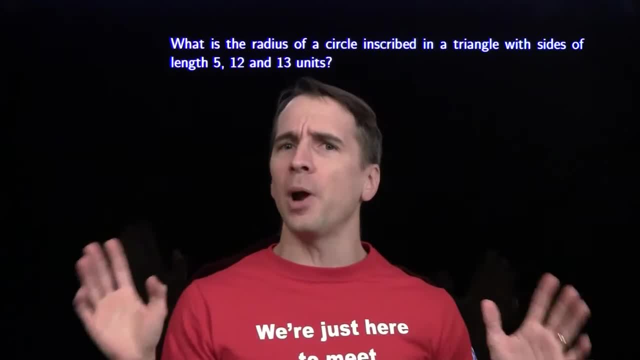 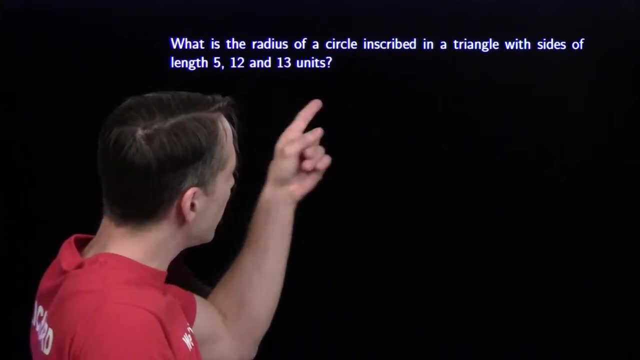 to talk some geometry. I'm going to show you my all-time favorite geometry problem-solving strategy: Draw a diagram, label everything you know, hope something good happens. I'm going to try that right here. We're looking for the radius of a circle inscribed in a 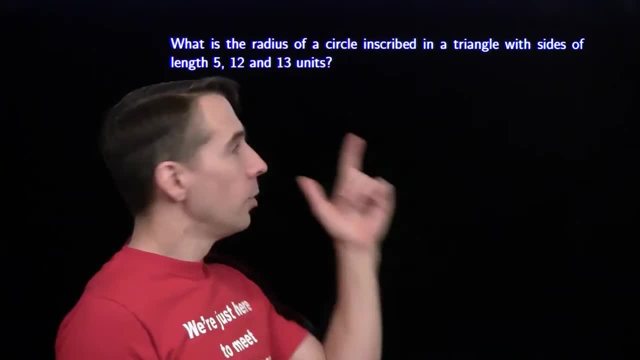 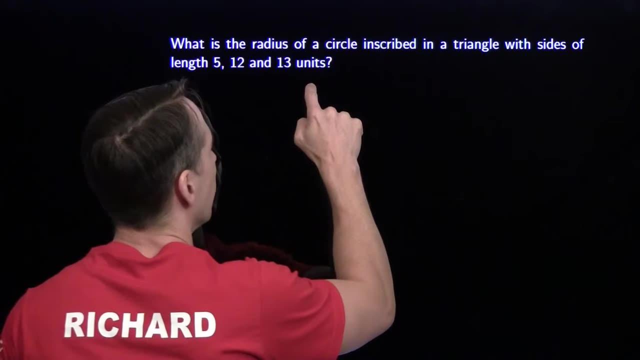 triangle with sides of length 5,, 12, and 13.. Well, we recognize these numbers right here. 5 squared plus 12 squared is 13 squared. This is a 5,, 12,, 13 right triangle. So we're going. 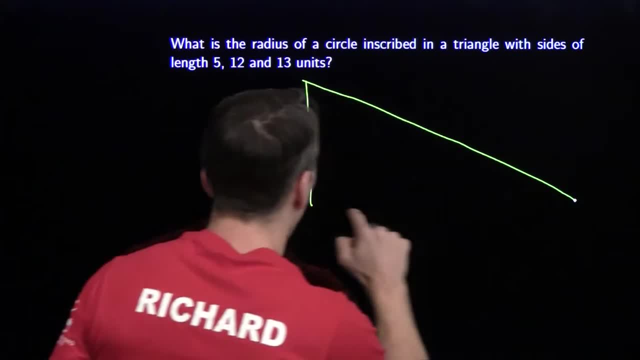 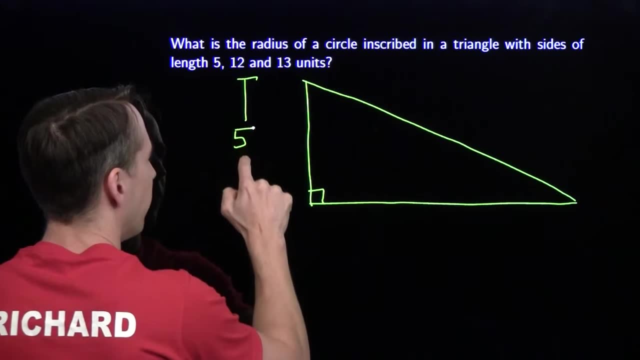 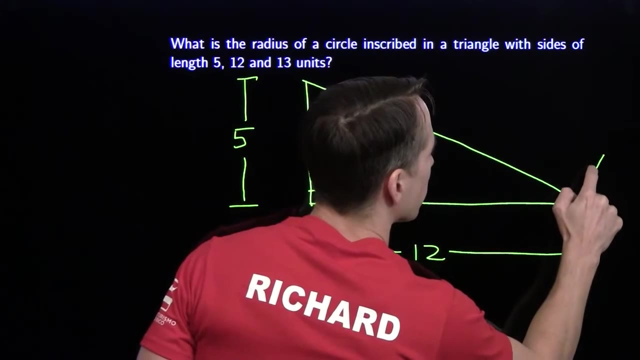 to draw a right triangle and then we'll label what we know Right triangle. very important to label that right angle. And we know that one of the legs has length 5.. One of the legs has length 12.. And the hypotenuse over here has length 12.. 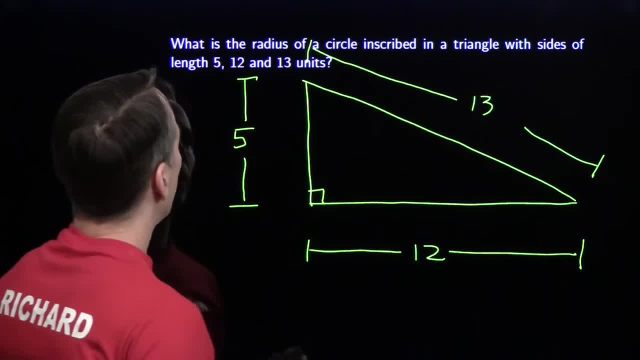 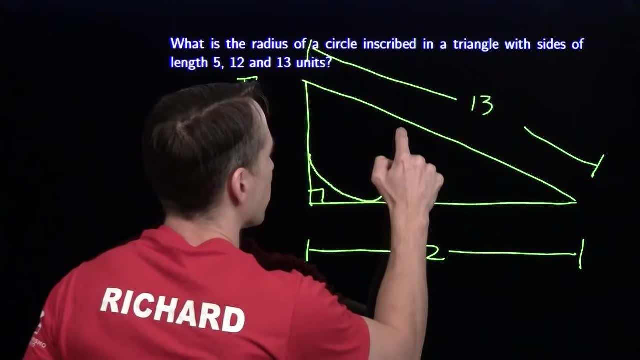 13. And well, we're looking for the radius of the circle inscribed in a triangle, so we need to add that circle in here. So there's our circle- Not a very pretty circle, but it'll do. And we're interested in the radius, so we need to add a radius to this diagram. 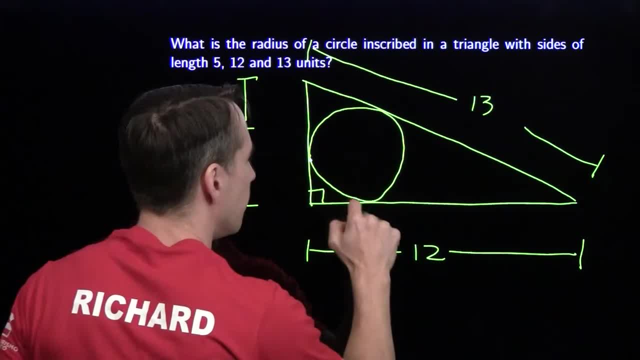 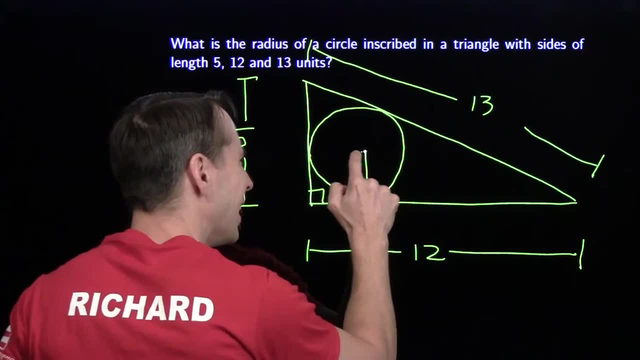 Now, a natural place to add radius is we draw it to the points of tangency, because the radius is perpendicular to the tangent at the point of tangency and we really like right angles. So we draw in those three radii and we see these three right angles. here We see, we've 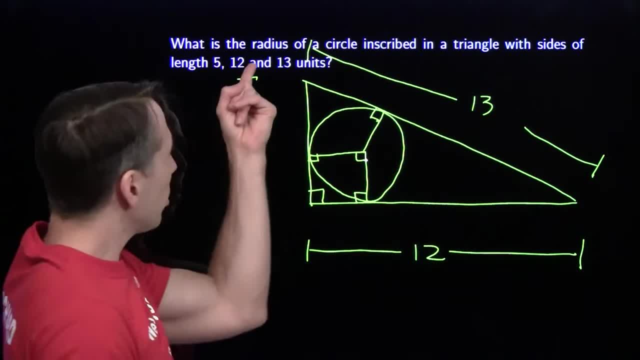 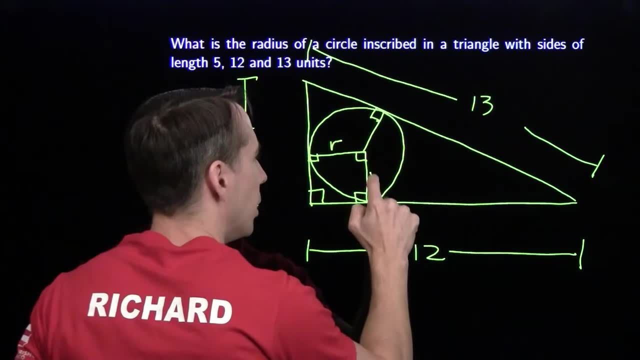 got a rectangle here. That's a right angle as well. Now we're looking for the radius. That means we're going to have to label the radius. We don't know what it is. That's what variables are for, And we're going to go ahead and add those to the diagram And as soon